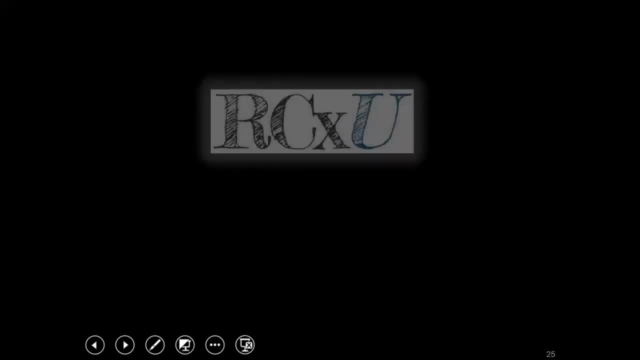 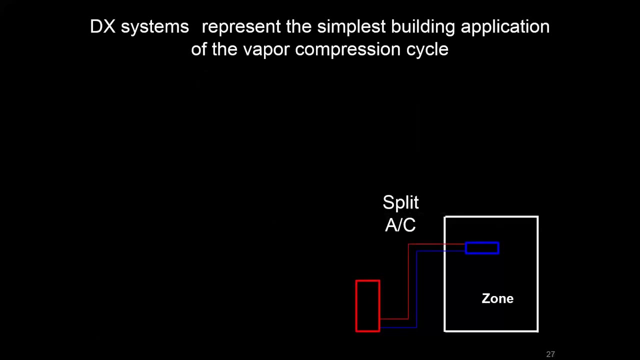 So we'll start out looking at air conditioning equipment by looking at a DX system. So this represents the simplest type of air conditioning system using the vapor compression cycle, And some of us may be familiar with an evaporator inside the zone and a condenser outside the. 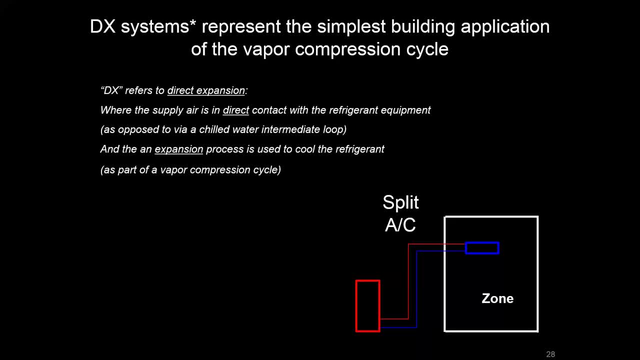 zone. So DX in this case refers to direct expansion, So the supplier is in direct contact with the refrigerant equipment, as opposed to something like a chiller that has chill water in between those two loops And the direct expansion refers to the fact that it's. 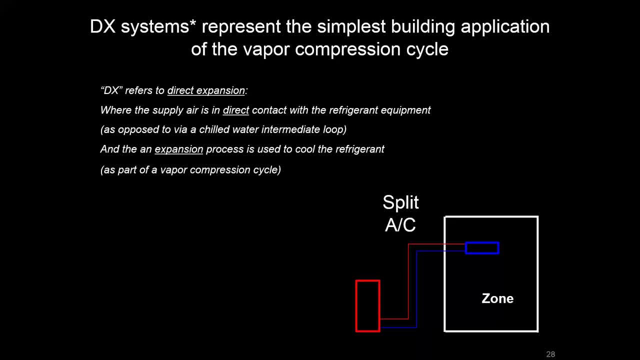 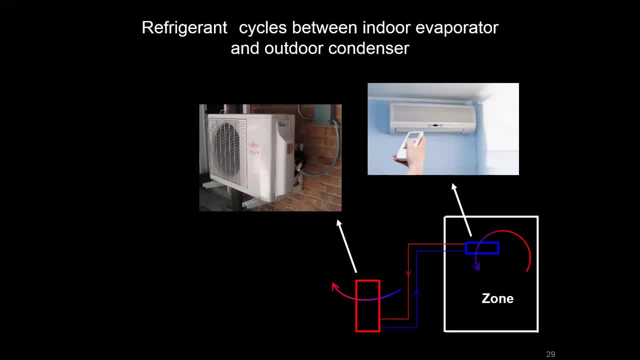 a vapor compression cycle which, as we'll see, uses an expansion process to cool the refrigerant. So here's an image of the evaporator and condenser equipment that we're probably used to. We're going to dig into that a little bit, But again, schematically, just try to think. 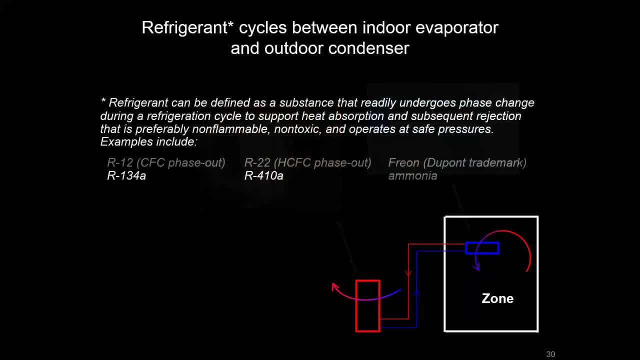 about those loops and how they interact with air. We define refrigerant in the last series in this way, and when we talk about refrigerant, we're talking about typically R134A or R410A, being pressurized, sometimes in a vacuum state, but sealed inside this loop running between the evaporator and the condenser. 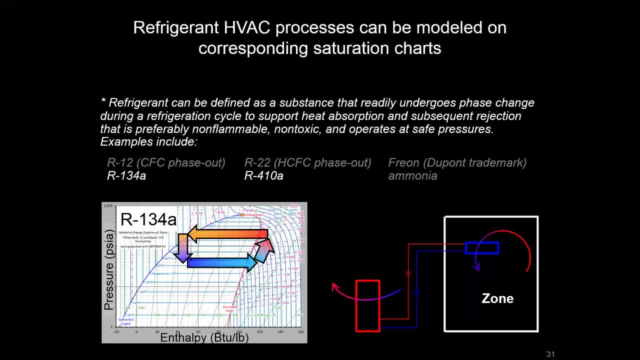 So we looked at the saturation charts last time for refrigerant, specifically for this reason, to prepare us for understanding and being able to chart this process as we look at how the refrigerant moves around this loop. So we're going to try to chart what we're. 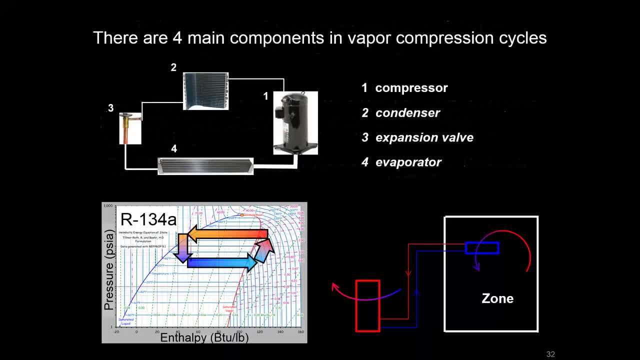 seeing schematically with what we see on the saturation diagram, And there's going to be four main components that we talk about in the vapor compression cycle. So the first is the compressor And that's responsible for pressurizing, the evaporator And that's responsible for the 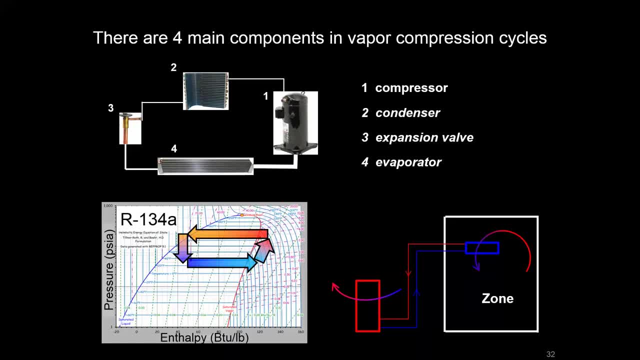 pressurizing the refrigerant in this loop and moving it around. As a byproduct, there's going to be a little bit of heat added as well. Let's keep that in mind. The second location or piece of equipment that's going to see this refrigerant is the.